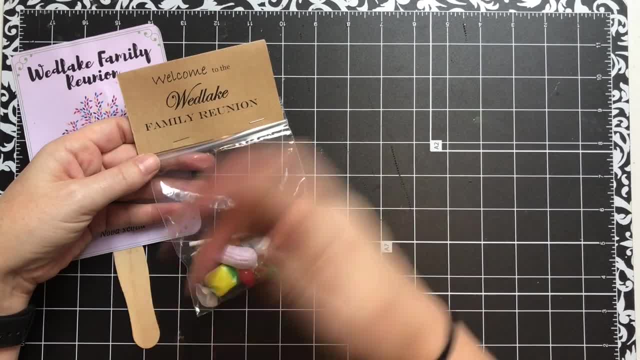 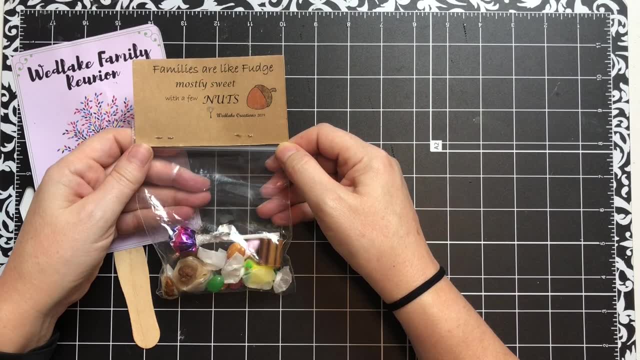 on top and we just stapled it. So it just says welcome to the Wedlake family reunion. And on the other side it says families are like fudge- mostly sweet with a few nuts. And then we put Wedlake Creations 2018.. So 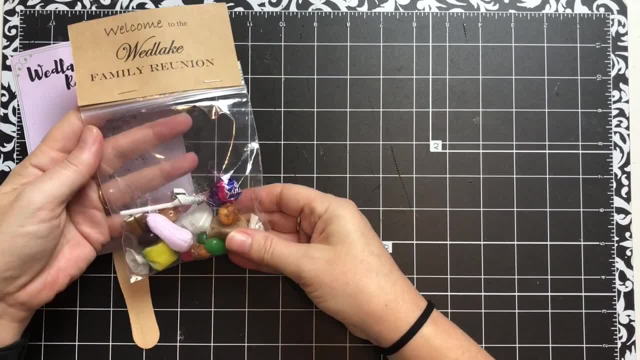 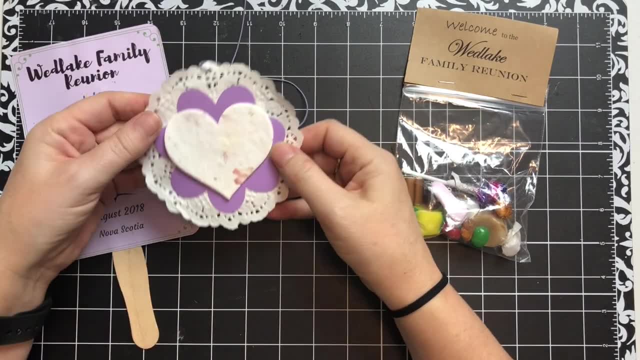 we thought that was pretty cute and nice little treats in there. So that's that one. Let's move that out of the way. Our next one is this little heart, And then I cut out with a punch- Actually it was a die. 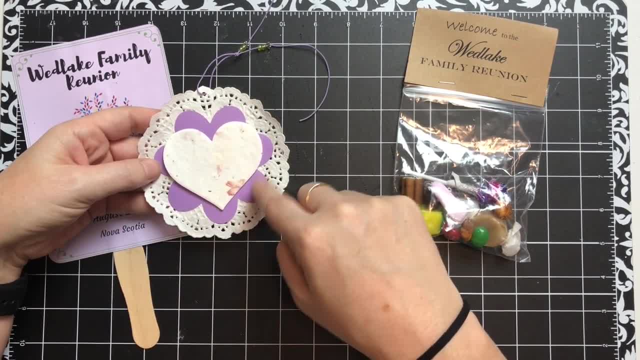 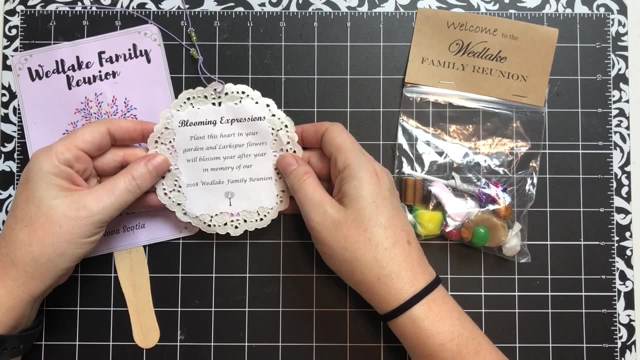 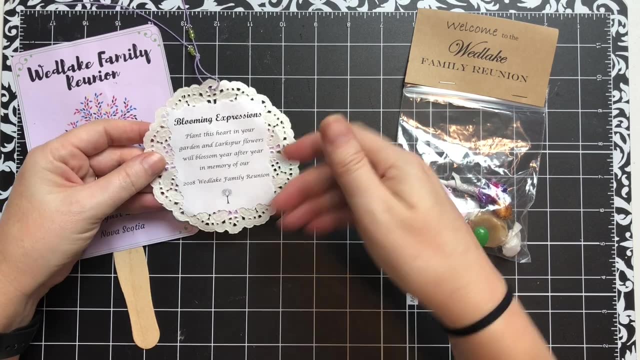 Okay, so that's that one, And then I cut out with a punch- Actually it was a die That we used- and just a little doily. So on the back we put blooming expressions. plant this heart in your garden, and leftover flowers will bloom year after year in the memory of 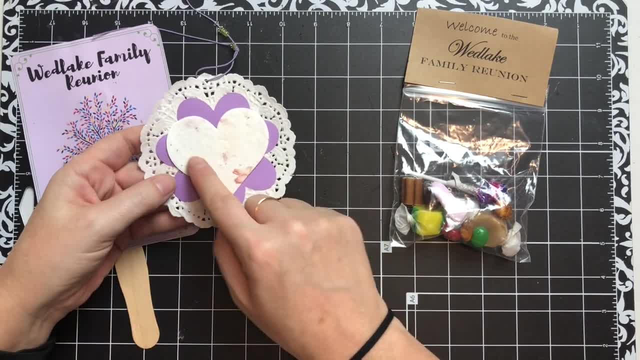 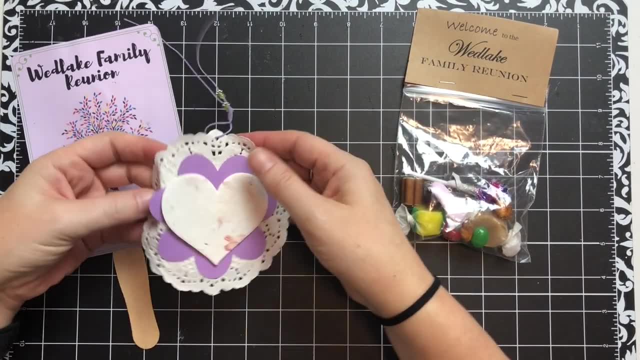 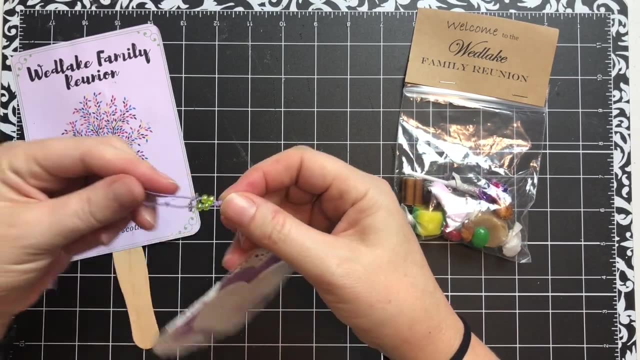 and we put the family reunion. So this little heart, you can actually plant it and it will bloom. So we made a bunch of these And then we just put some of the little ribbons, of the little ribbon here, and we just put some embellishments on little beads and that on it. 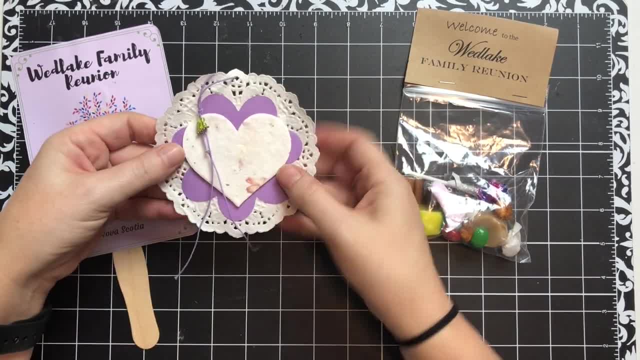 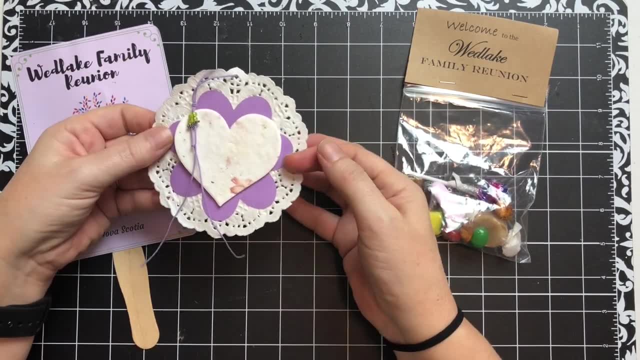 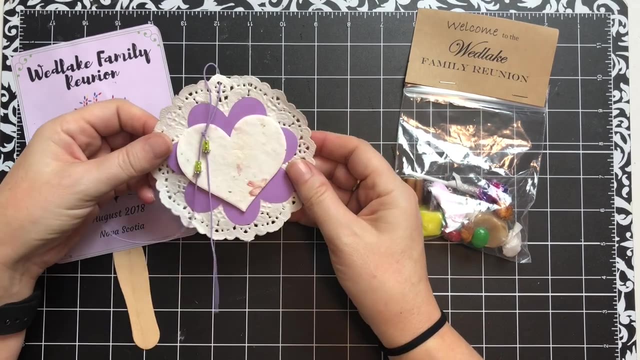 thought that added a little twist to it, and so they can bloom. they sorry plant just this heart. and then, voila, i thought it was a great little idea. you can reuse the the flower piece if you wanted. um, if someone like doesn't like throwing stuff away, and the doily could be used for your. 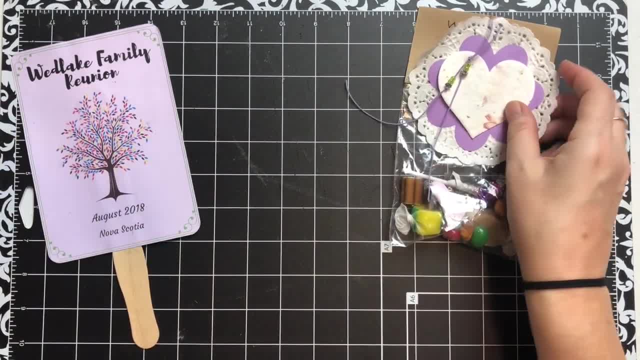 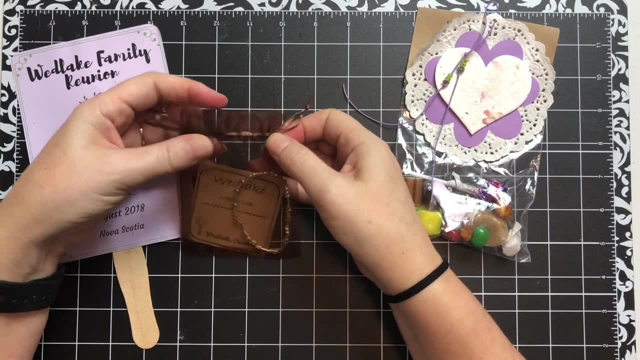 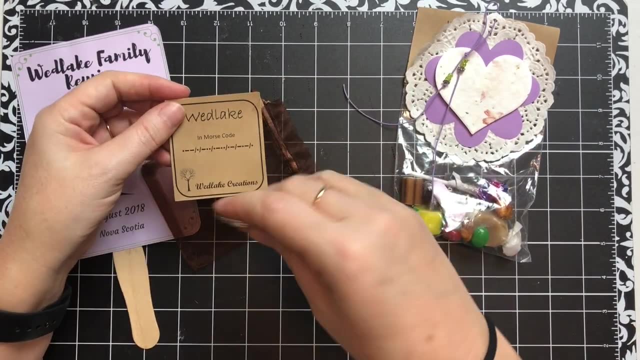 tea or coffee at home and you know everything can be used. so we have that. and then this one was a really, really creative idea. i saw this on pinterest. i saw it in several different spots, but this was really cool and unique. so we did a bracelet in the family name in morris code. 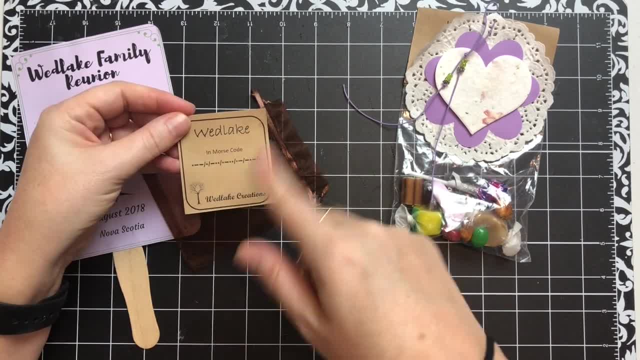 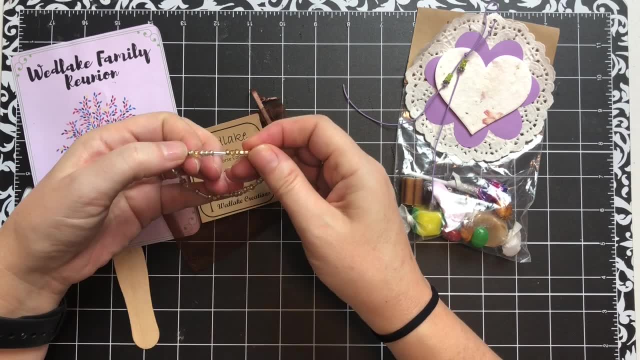 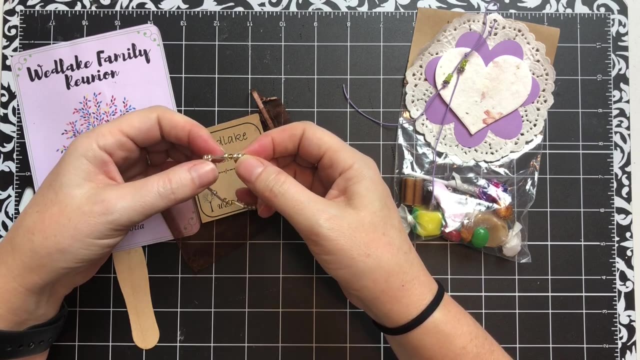 so, uh, it would be wed like, and every slash, you know it was between each letter. so this is this, is it here? so the longer space bars, we use that as a slash, and then we use silver, uh, for the- i think these were for the dots- and then we use the, um, the gold.